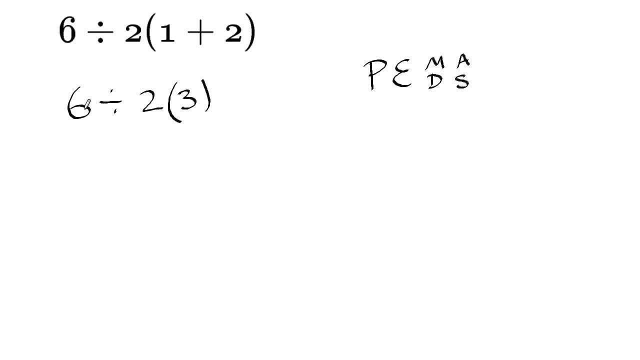 this one's to the left, so that one happens first. So you do the 6 divided by 2, and that makes 3, and then that's multiplied by the 3.. So now we do that and that makes 9.. So let's see how the order of operations applies to something like. 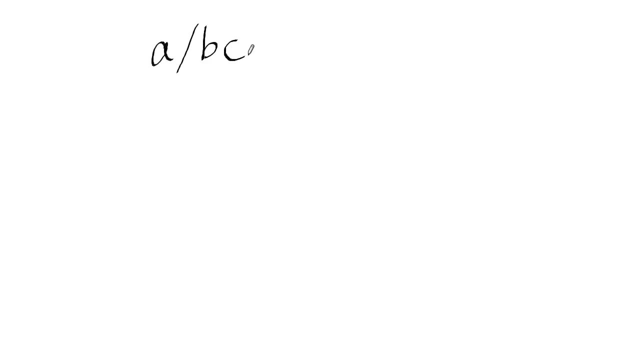 A slash BC. So again we've got a division and a multiplication. we start on the left. so A divided by B is the first thing you do and then you multiply result of that by c. So this, according to PEMDAS, is the same as a over b times c. 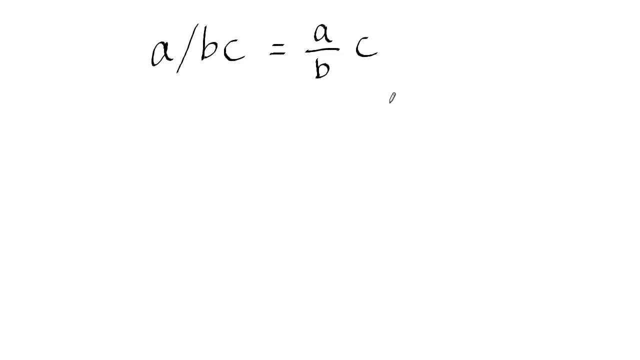 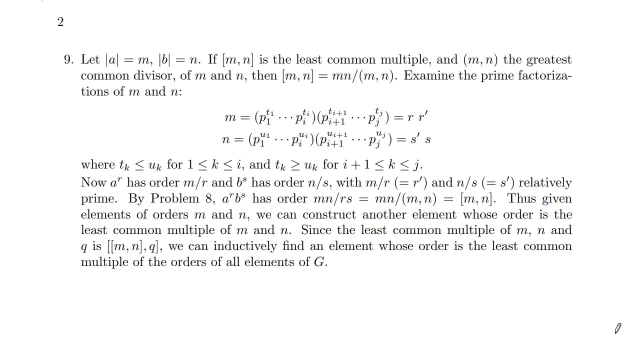 But is that how mathematicians, scientists and engineers would actually interpret this expression? So to test this out, I just googled mathematics textbook PDF and this is the first one that I clicked on. This is abstract algebra by Robert B Ashe And you can see on the second page of the PDF. I just 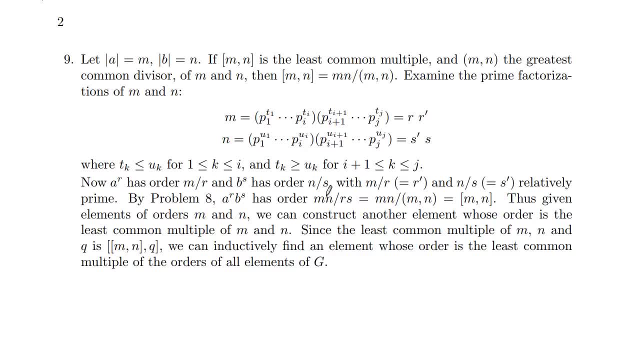 went straight to the, the answers to exercises, because that's where I was expecting to find expressions like this. So we've got this, what they've done to get. that is multiplied the m over r by n over s, so that would make m n over r s. 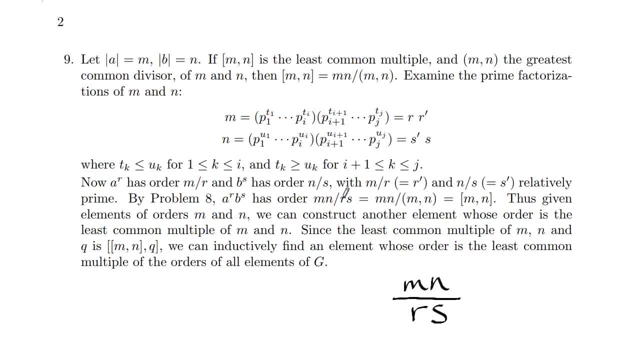 And then they've written it like that, though, whereas the order of operations would tell you that that means mn divided by r. the division comes first, and then you would multiply by the s, and that of course makes mn s over r, But they're using it to mean that, so they're obviously not. 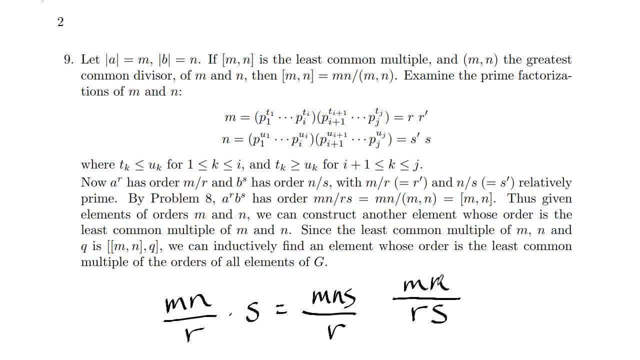 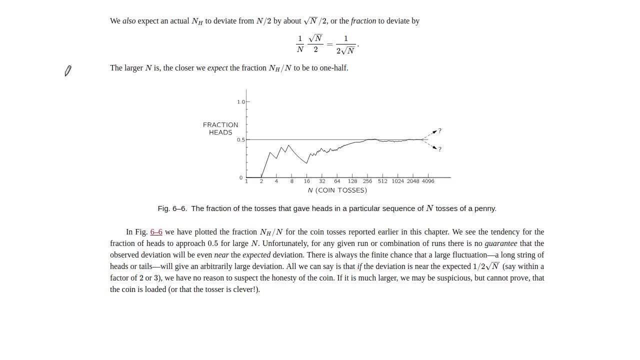 using the order of operations as it's taught in primary school. What about physics? This is from the Feynman lectures on physics. We've got a deviation of 1 onto root n and then they've written that again down here inline as 1 slash 2 root n. Now order of operations would say that: 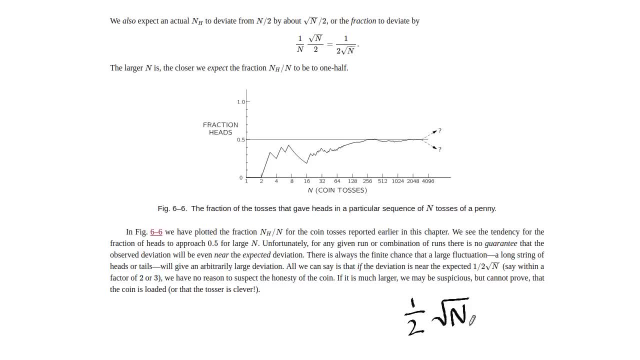 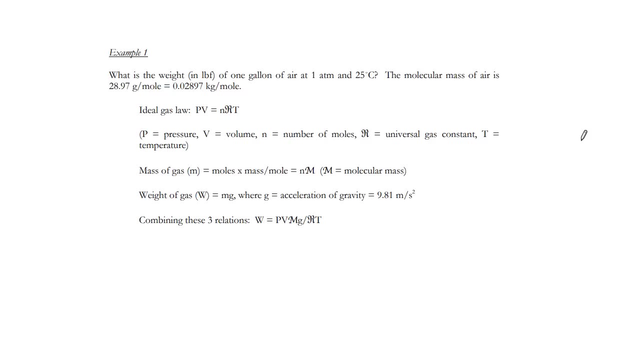 that means half root n, but they're using it to mean 1 on 2 root n, so they're doing the multiplication first before the division. What about engineering? I've just Googled engineering textbook pdf and this was the first one that I clicked on. This is on on page 15.. I'll 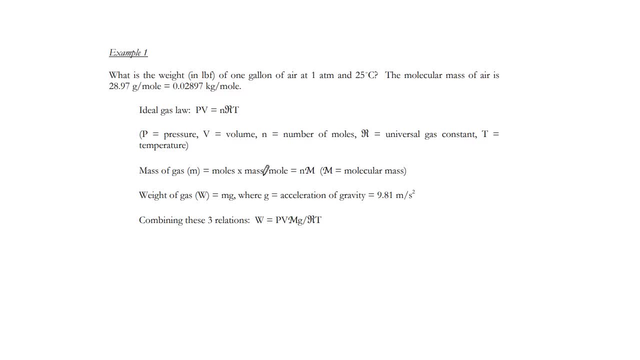 put a link in the description for the left-hand side of this. I'll put this link in the description here as well. I've got all of these quantities in the right hand portion and then these two to it in the description. but what they've done is they've solved these equations for w and got pvmg. 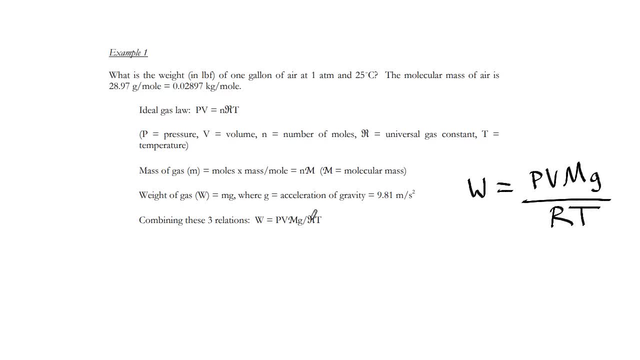 on rt, and then they've written that like this, with a slash: rt and PEMDAS would say that that means pvmg divided by r, and then you would multiply by t, and that is not the same thing as that. so they're not using PEMDAS, So the textbook authors aren't following PEMDAS. 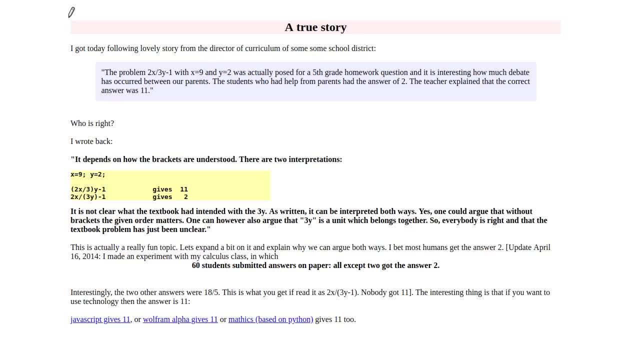 but what do the students think? Well, Oliver Nell of Harvard asked his calculus students this question: what is 2x over 3y minus 1, if x equals 9 and y equals 2?? Well, according to PEMDAS, you would say: 2 times 9 divided by 3 times 2 minus 1, 2 times 9 is 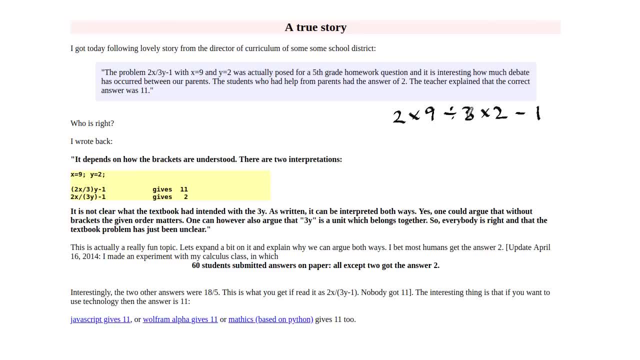 18, then you divide by 3, that makes 6,. you multiply by 2, that makes 12, and then you subtract 1, that's 11, and this is what this 5th grade teacher was saying. They asked their. 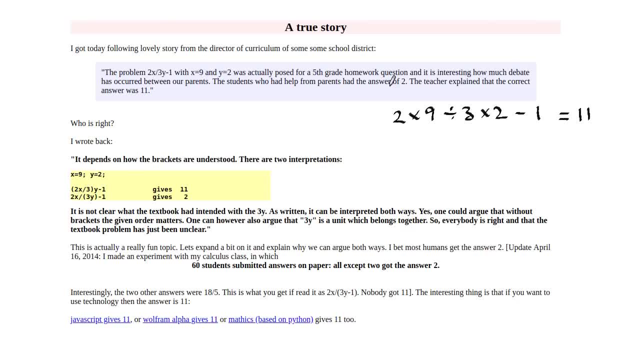 students this question and it caused a bit of a stir because the parents and students didn't agree. So, in way, Oliver Nill asks his calculus class this question and 58 out of 60 of them said no. it's 2 times 9 over 3 times 2, and then you subtract 1, so that's 18. 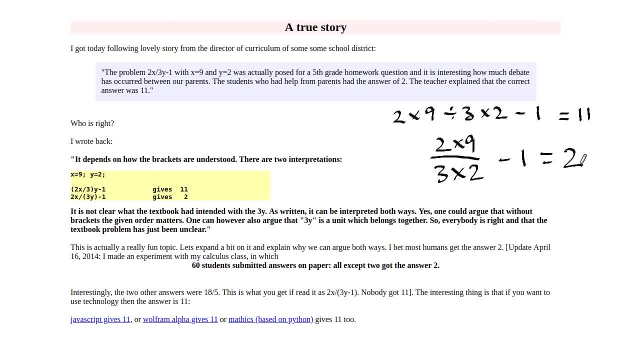 over 6,, which is 3, and then minus 1 makes 2.. 58 out of 60 said that The two that didn't, interestingly, didn't say 11,. they did 2 times 9 over 3 times 2 and. 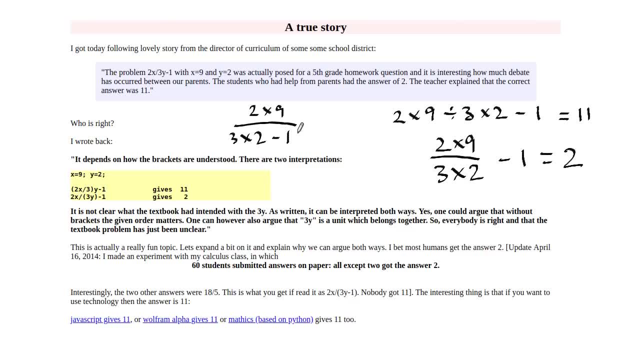 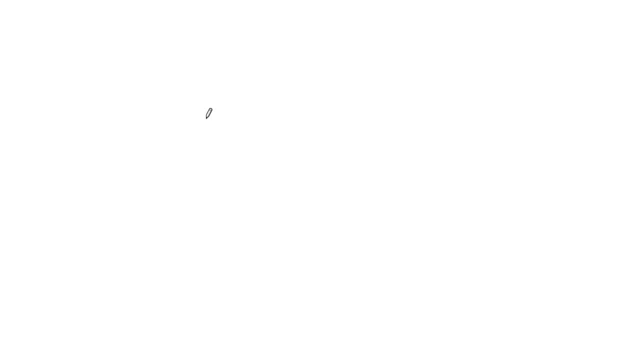 put the minus 1 in the denominator as well, So absolutely nobody would interpret the question like that. It's easy to see why this became a rule. If you want to write something like 1 over 2x in one line, you would have to use 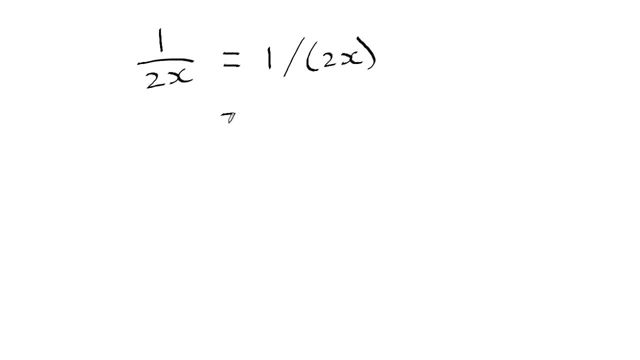 brackets, which is annoying. So mathematicians tend to be quite lazy and they just write 1 slash 2x when they mean 1 over 2x. So that's the problem. Now, the order of operations that you would learn in school says that this is the same as half of x. 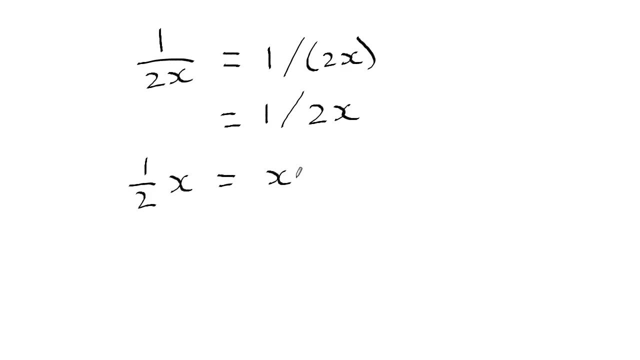 But there's a much easier way of writing this: You could just say x over 2.. So people have developed this rule that 1 slash 2x means 1 over 2x, and if you want to write half x, you just write x over 2.. So it's an unofficial rule that's used by almost everyone in math. 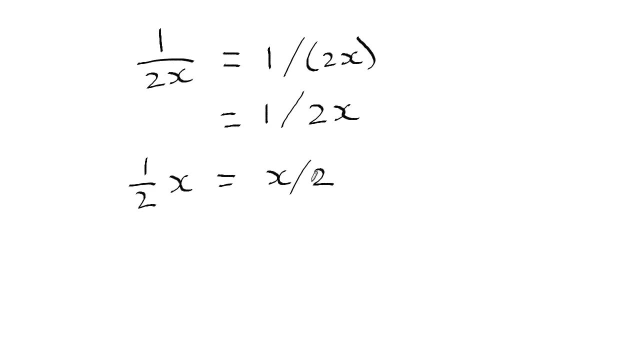 science and engineering. But has it ever been an official rule? Well, indeed it has. This is from a style guide put out by the American Mathematical Society, and here they clearly say that they use the rule that multiplication indicated by juxtaposition is carried out before division. And here they're just saying: 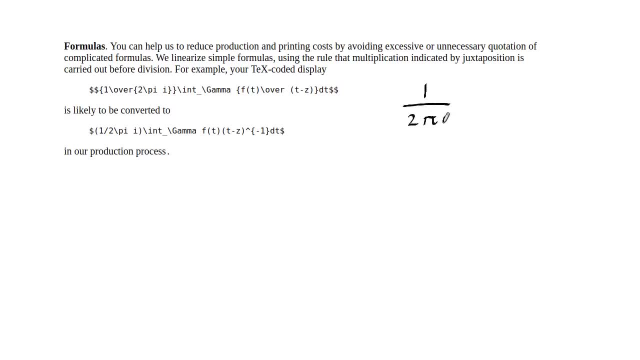 that if you write something like 1 over 2 pi i, they're going to change it to 1 over 2x, 1 slash 2 pi i, and that these mean the same thing. Likewise, the American Physical Society. 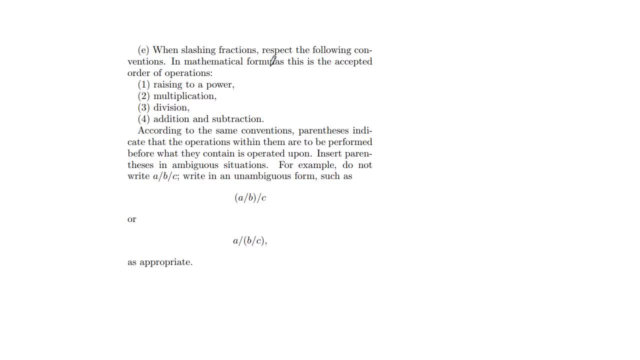 in their style guide, say: in mathematical formulas: this is the accepted order of operations: raising to a power, then multiplication, and then division, and then addition and subtraction have equal precedence. So how does this rule apply to our question? Well, you still start by. 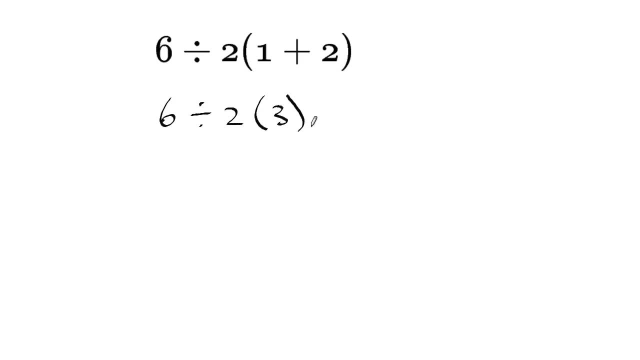 evaluating the order of operations. and then you start by evaluating the order of operations. What's in the parentheses? That makes 3.. But then multiplication by juxtaposition comes before division. So we've got 6 divided by 6, which makes 1.. So although PEMDAS says